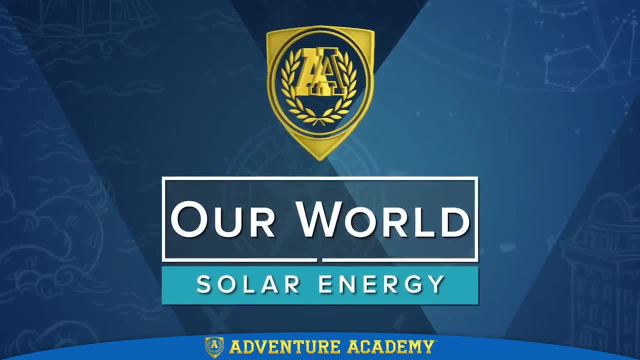 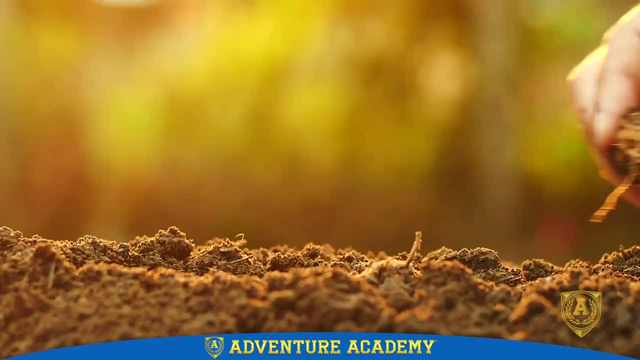 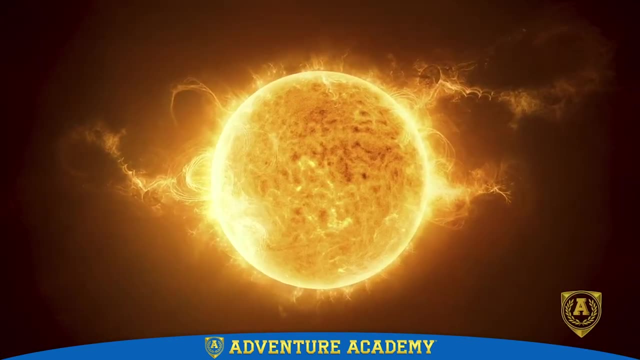 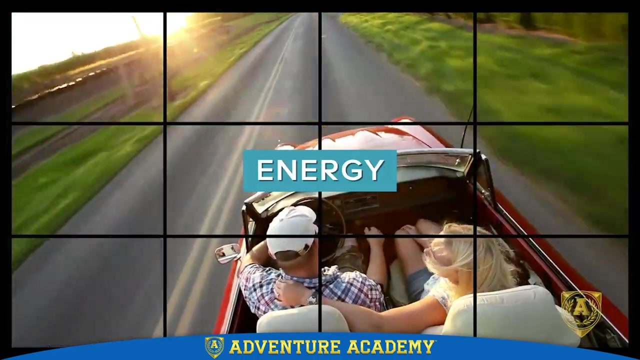 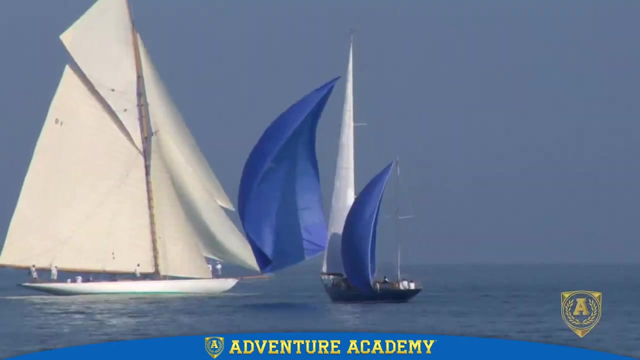 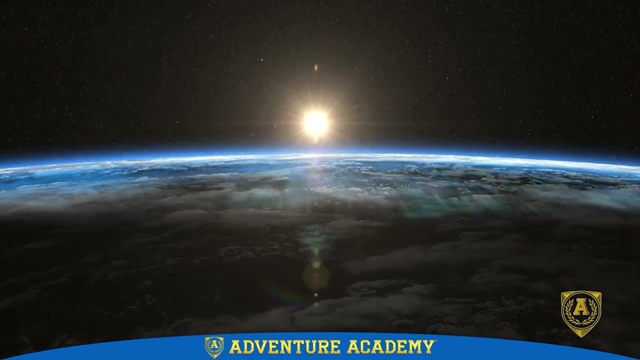 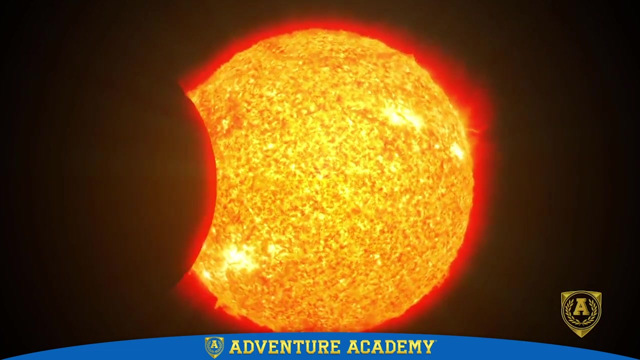 Thank you for watching. Energy is everywhere and takes many forms. The heat and light that comes from the sun can be harnessed and turned into other forms of energy that we can use. When we talk about things related to the sun, we use the word solar. 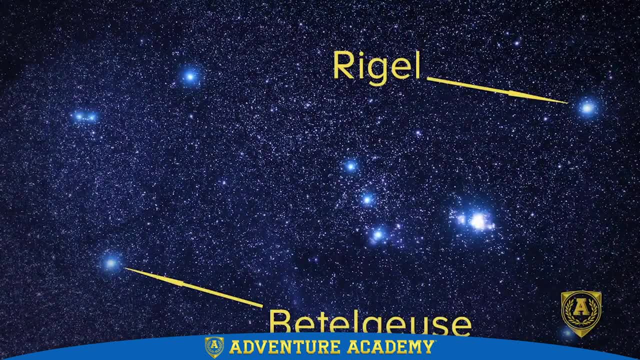 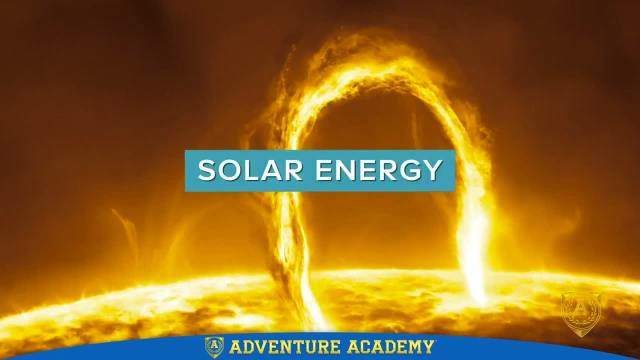 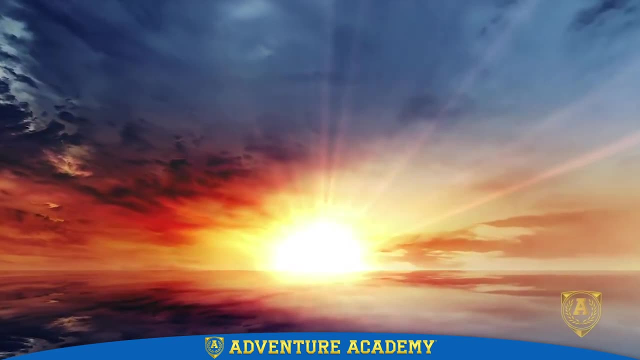 That's because our sun, like other stars, has a name. That name is sol, and the word solar comes from that name. Solar energy is constantly flowing and won't run out for billions of years. Any source of energy that can't be used up is called renewable energy. 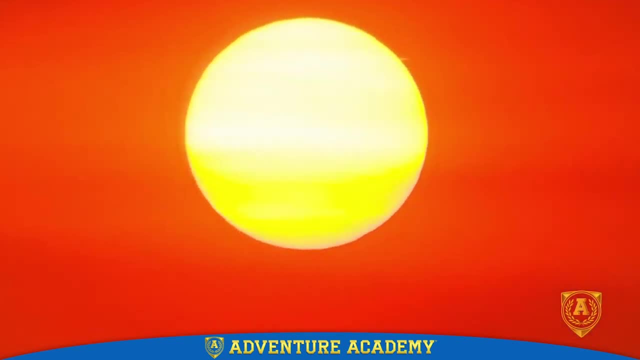 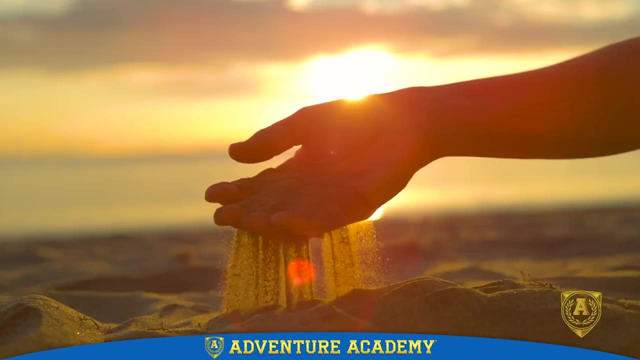 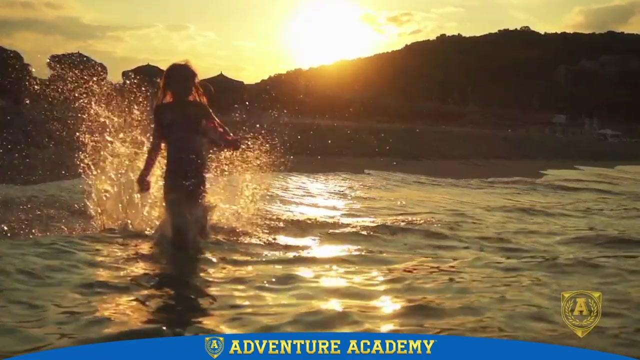 Let's look at some of the ways this wonderful source of renewable energy can be used to better our planet and our everyday lives. When solar energy hits objects on Earth, it turns into heat, and this heat can be used to keep us warm and comfortable where we live and play. 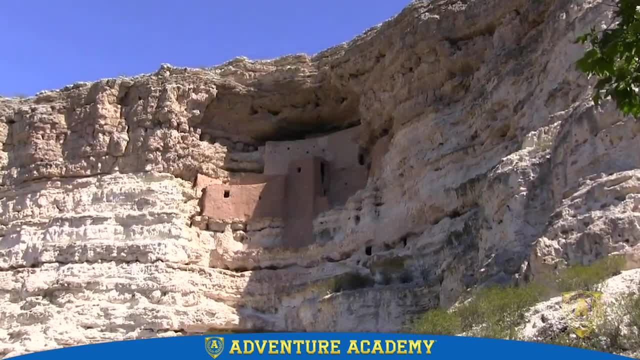 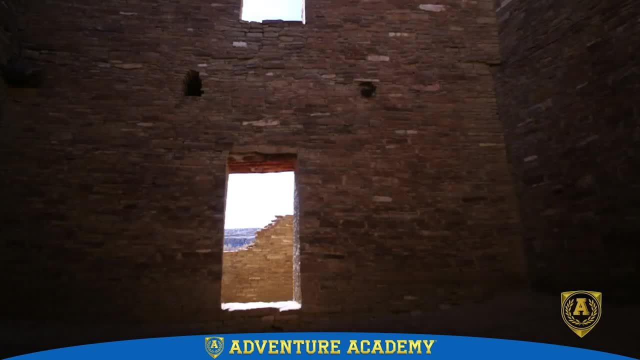 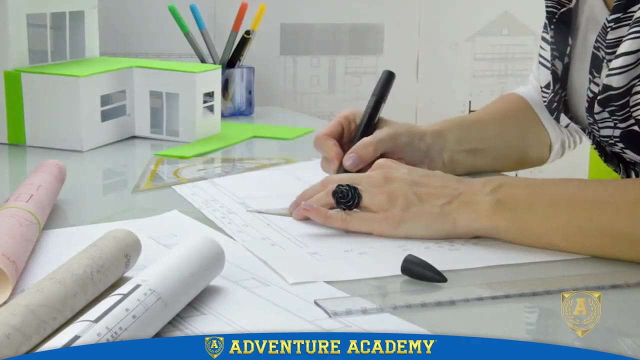 Ancient cliff dwellers said, and Arizona took advantage of this almost 1,000 years ago By positioning their homes so that the winter's sun would shine directly inside. they used this natural resource to make their dwellings more comfortable. Today, people design homes and offices in ways that take advantage of the sun's warmth in winter. 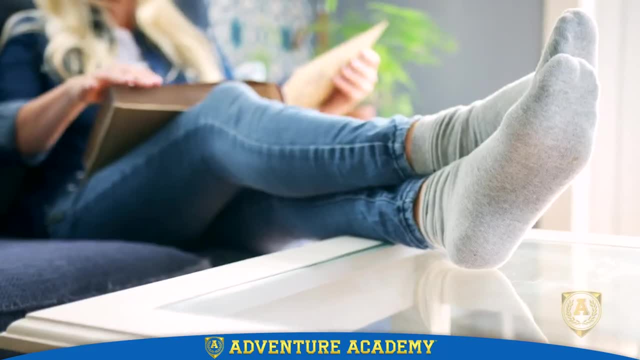 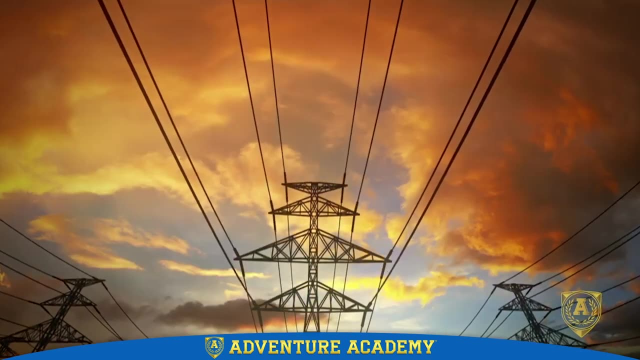 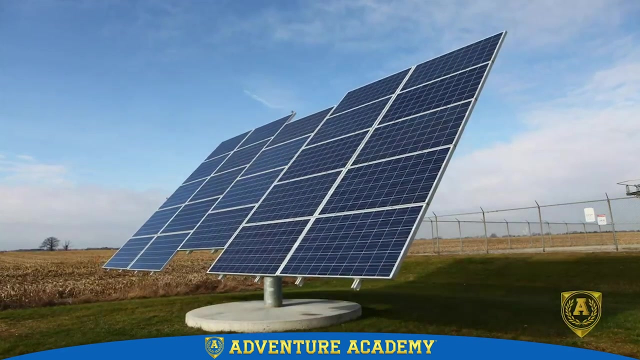 or shield us from its heat in summer. This not only makes people more comfortable, but also cuts down on the costs of heating and cooling. People have also created ways to use solar energy to generate electricity: Panels built with light-sensitive elements and positioned to capture as much sunlight as possible. 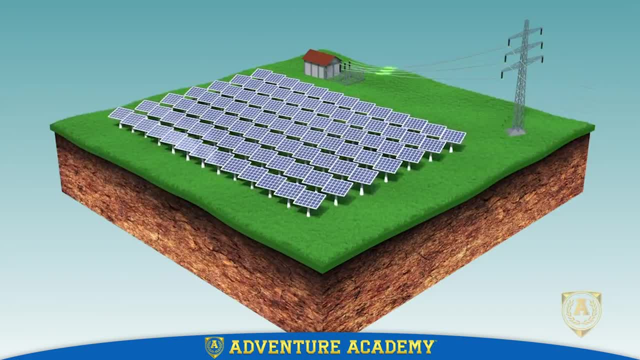 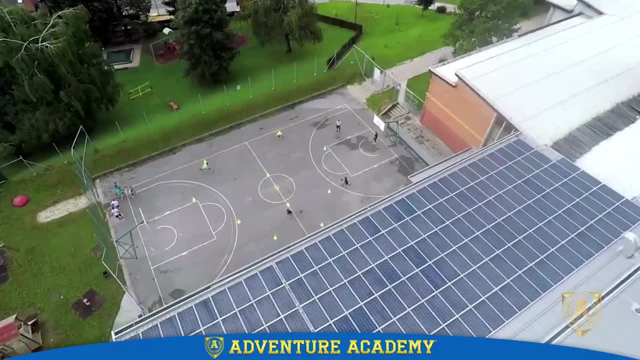 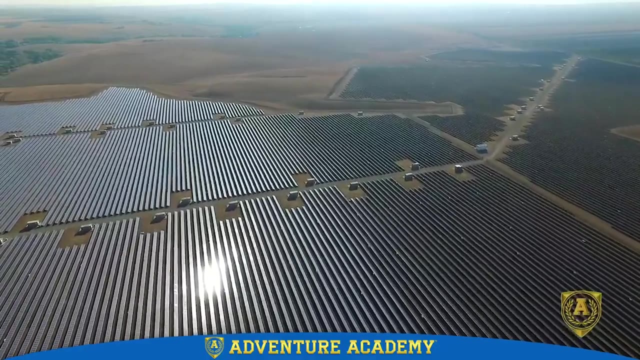 are able to turn solar energy into electrical energy. Small solar panels can power street lamps. Larger panels can power homes, schools and office buildings. Solar panels that are spread out over large areas are called solar farms, and they can provide enough electricity to power a whole lot of people.